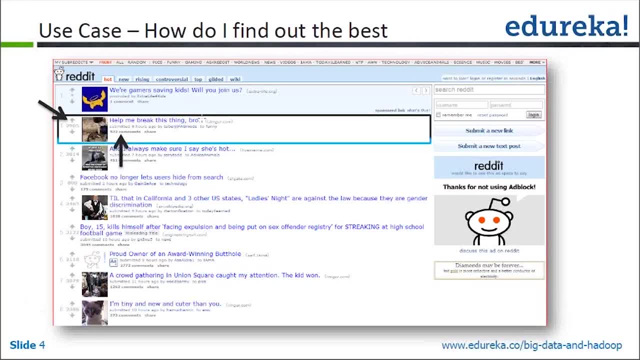 So basically take all these, the activity which users are doing on this particular site and then, based on that particular, the log which I'm able to get from the users activity, Give me the top 10 links, like: which are the links which will be used by the you know, by a particular you know, sorry, which are the top links which are used by the users, Right? So that's all is my requirement, and I need a big data solution for that. 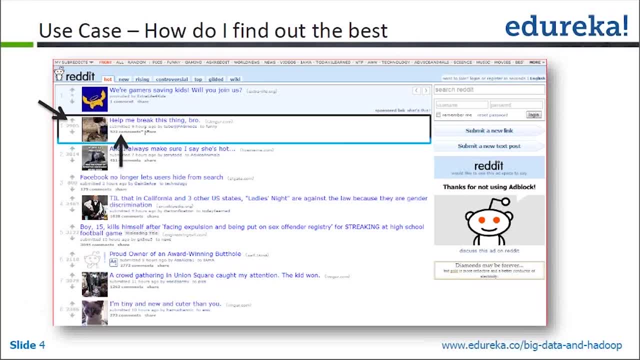 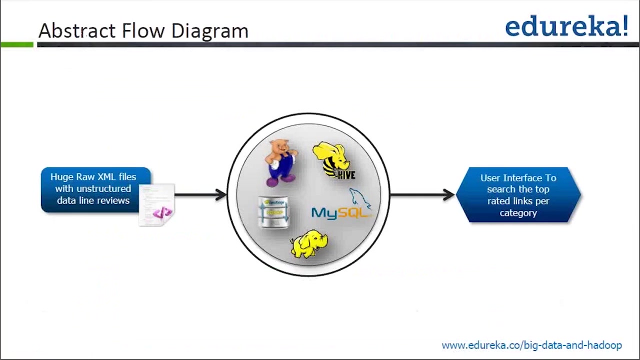 Because I know that the volume of the data which I'm doing here is use volume of the data. So, based on, you know, this requirement and you know I want a big data solution and this is my problem statement. I would leave it to you guys to ask any question which will you will need to answer in terms of implementing this project, Okay, Okay. So here is the thing, guys. So what we have is like, we have the data set, that is basically XML. 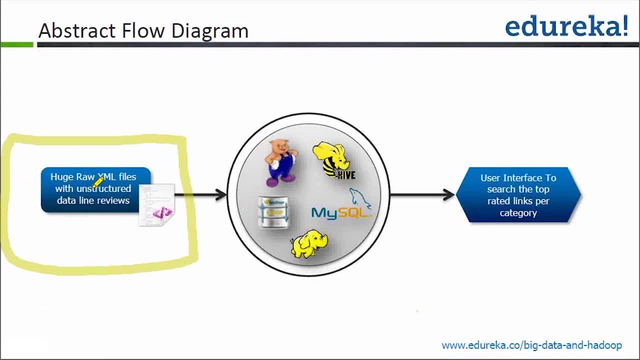 That is available at the XML data set And that's basically the use of, you know, the XML file which we are getting from the site. Now what you have to do is you have to basically get this data inside Hadoop. So that's the first step. So how you are going like to approach most of you you know, like you know, give here is like whenever you have this Hadoop kind of the problem, the first thing what you will do is you will try to understand what kind of the data you are going to use. 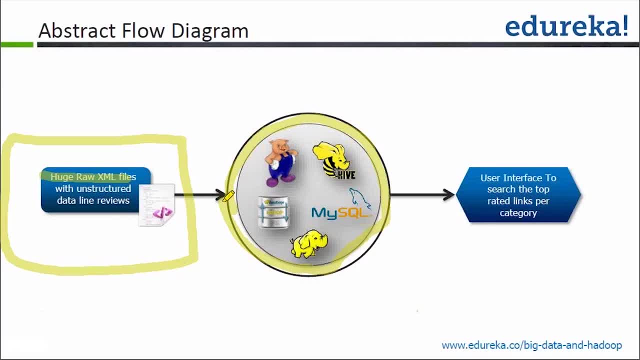 How you are going to process. So right, Because your whole set of tools, the flow, everything is going to be determined based on the, based on the kind of, you know, the data you have. So, if you have structured data, you are going to set one set of tools. You have uninstructed data, another set of tools. So it's so. it's very important, like the next time when you start your discussion about the Hadoop project, just don't start like, okay, I'm going to implement the MapReduce and I'm going to talk about the ping. First have a cup of coffee with your client. 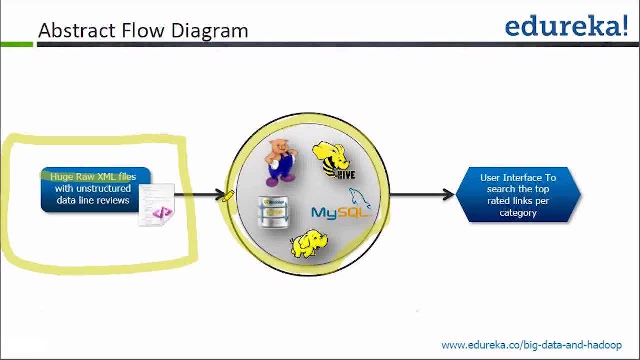 Or whoever giving you the requirement and ask them: okay, Hey, tell me about your data, set, What kind of the data you want us to process, Right, And then try to understand whether the data is structured data, uninstructed data, semi structured, and based on that, you ask the next set of the question: Tell me, like, how you are going to make the data available. So, is it like that the client is going to send you a file and that's the way you are going to consume the data, or is it the data is going to be available through some API call- XML data- or is it available in some RDS? 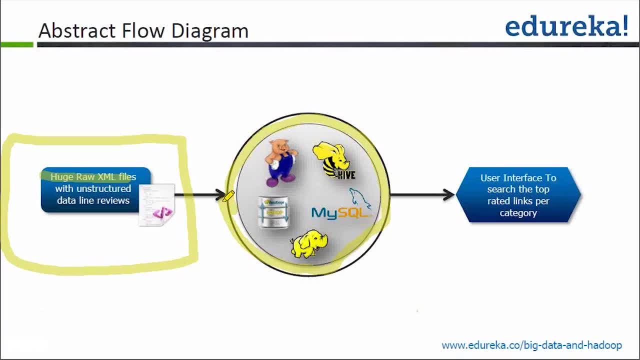 Maybe in a stable, and that's what you have to go in fetch. So, based on these information, what you do is you decide the strategy, like how you will bring that particular data set inside the Hadoop Right And based on that, you decide to bring the data in Hadoop. And once you decide that particular strategy, then you go for the next level of approach, like we will decide how to process the data. And that particular stuff you will do is like based on understanding the business requirement, what they want to see from the data, what the data is available and what kind of the competition you to do. 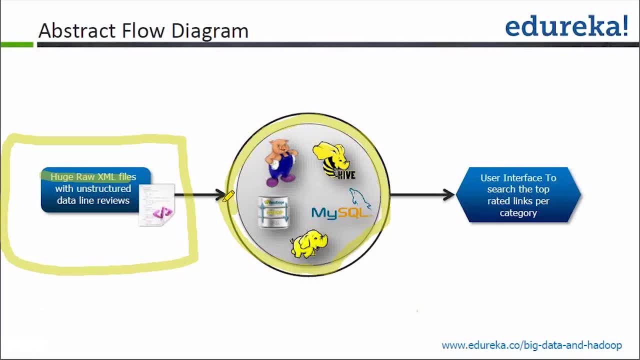 That you will decide the implementation part and based on the implementation and the kind of the data you have, you will go for like option, like whether I should go for big, I should go for high or I should go for directly MapReduce coding. So that will be your next level of strategy And once you decide on the tool, then you go is like how you are going to expose this data to the client. 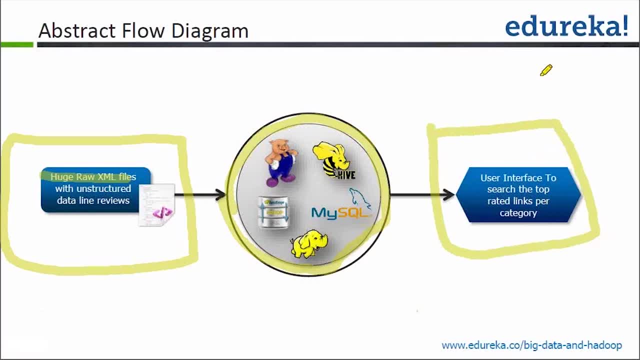 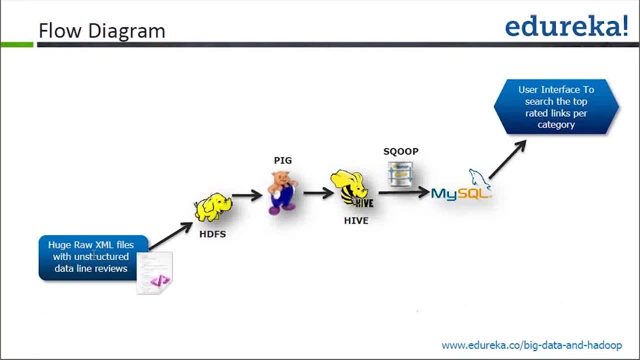 Right, So that will be this user interface part, like how you will present this data to the client. So this is a kind of a one flow, guys, where you have the huge XML file that you want to process as part of this Hadoop processing and then you move first. what you do is you bring the data inside Hadoop. so that's what you have. you bring in the data inside the Hadoop processing, then you use a set of tools- maybe MapReduce, BigHive- you can use that- and then like, if you want like to present data. in our case we wanted to see a report where we wanted to have like top 10 records. 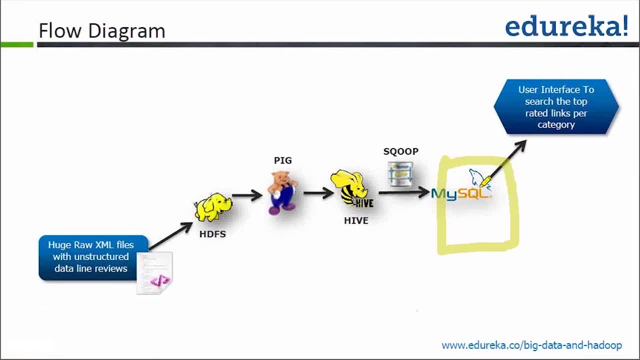 So in that case, what you can do is you can have your report tools and that can connect to the database. so so what you can do is you can move this data from Hadoop to any kind of RDBMS system and that can basically enable your reports to connect. that and do the, you know, the faster. 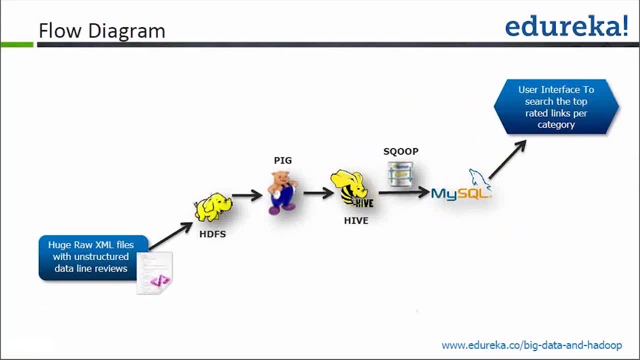 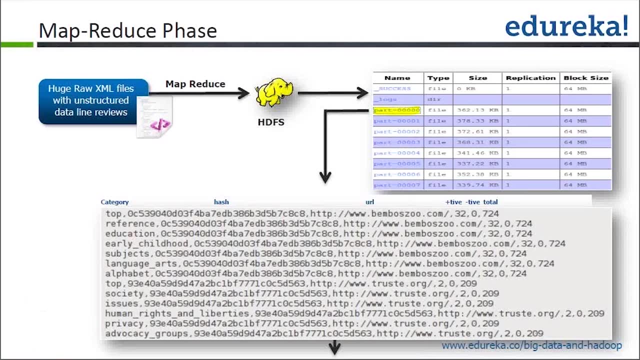 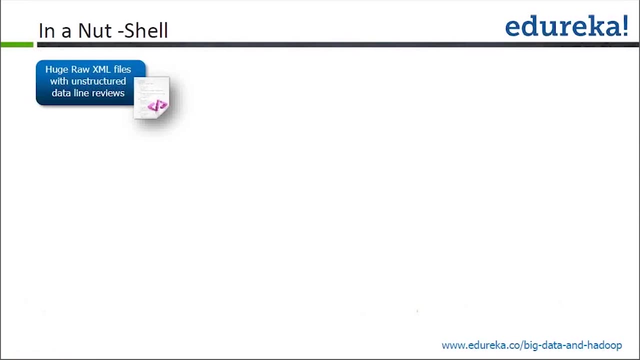 reporting from there. we'll see the more details here, guys, for this whole implementation. right, so you can go, go through the different phase, like the MapReduce phase, big phase, in a high phase you can. you can go through and then that's where your data will be exposed. so in a nutshell, right, how you. 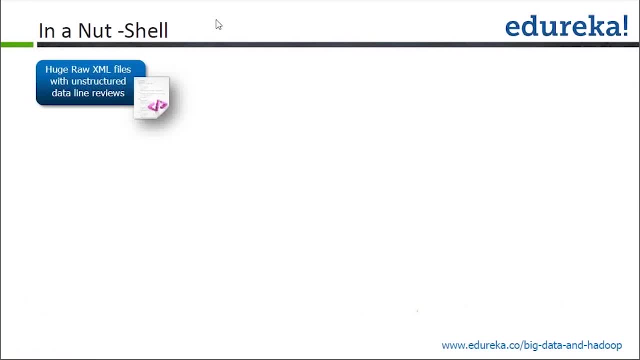 are going to basically output this stuff is like you will have this huge XML data set that that's what you are going to get from. you know that, from the user or the client, and then the first thing, what you will do is you will bring this data. 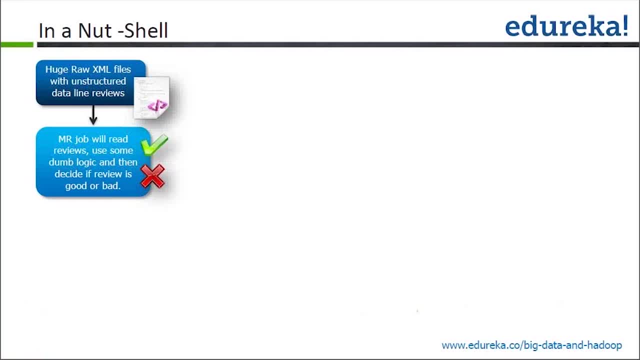 set inside HDFS. so sometimes what will happen? the data set will not win the appropriate format and in that case what you can do is you can use this map MapReduce job to basically bring some kind of a structure in that data, even if you want to do some kind of. 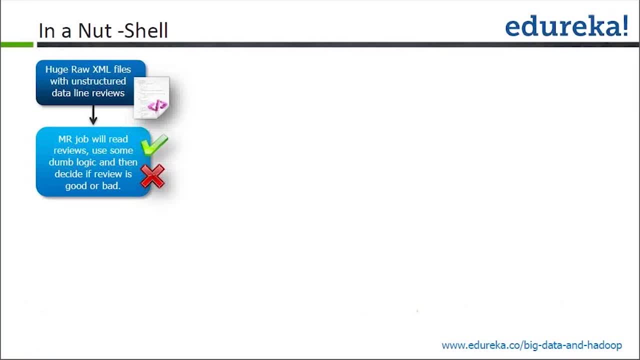 filtering or removal of the data. you can do that and then, once you have cleaned your data with the help of, like, whatever the MapReduce processing or, you know, in the peak for high processing you can, you will have a basically the data, which, in our case it was XML data. so you can, I like, have some XML data to pass the data. 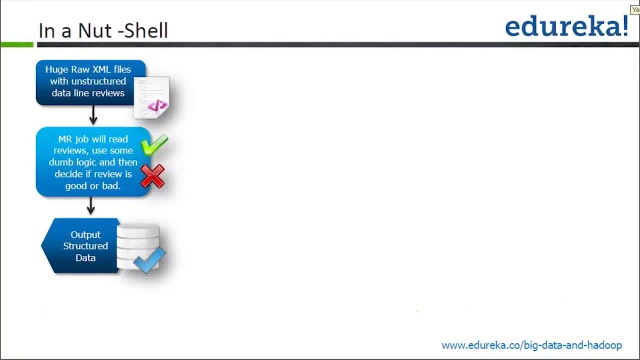 and give you the data in a structure, you guys, in a sector format. what you can do is you can use, basically, big kind of processing to get that is such a data and process that. so, like we wanted to have the, you know the rating of the data, what is the top, top, top and the kind of 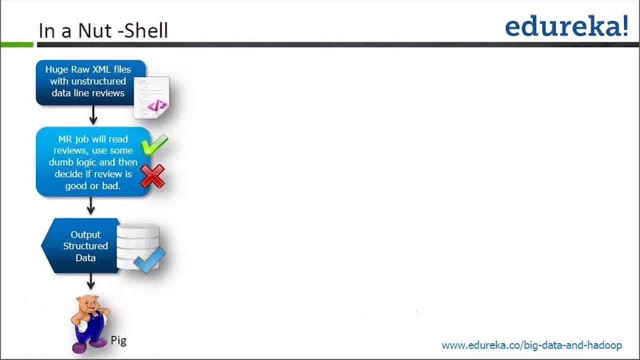 you know the URL, so all those kind of. you know the simplification or aggregation. you can do a bit like the combination of the pig and high processing so you can categorize your data, you can get add the rating and, if you want to- basically I know- see more details about the data or some more. 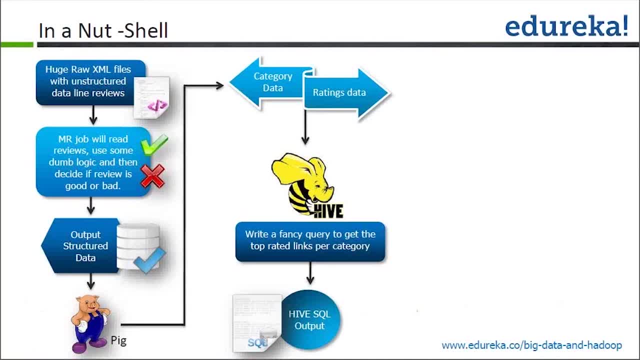 aggregation. you can use hive as well. so by using the hive query you can see like top 10 record. so give us the top 10 record based on the URL value. you know you can summarize that and you can do that once your data is available as the 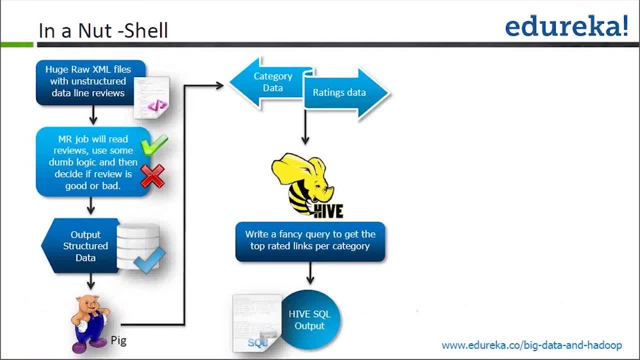 aggregated data and you need it for the reporting. so what you can do is you can output this data set to any kind of the RDB, my system, and that's the way generally people do the reporting on top of Hadoop, because Hadoop has due to it. 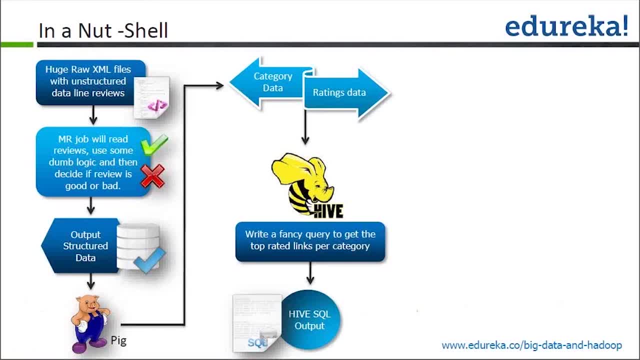 like the. you know the kind of the Hadoop system. you know the kind of the Hadoop system. you know the kind of the Hadoop system. you know the kind of the system is built when it comes to consuming the data, like from hive and all. it's going to have very high latency because it's it's a kind of- you know the. 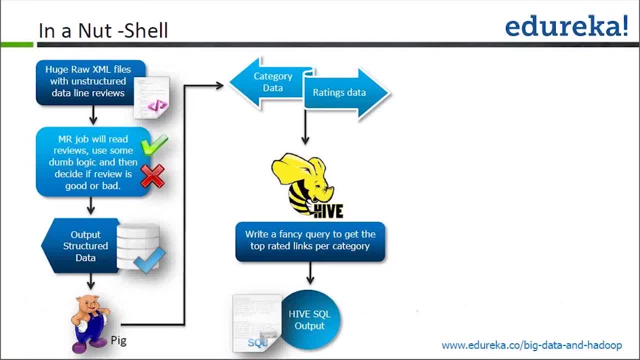 MapReduce application which it is going to run to give the data. so for reports you you need, basically for the users, low latency report. so what you do is you expose all this data which you get from the Hadoop aggregation or Hadoop processing in into some kind of the RDB message structure. may be like tear data. 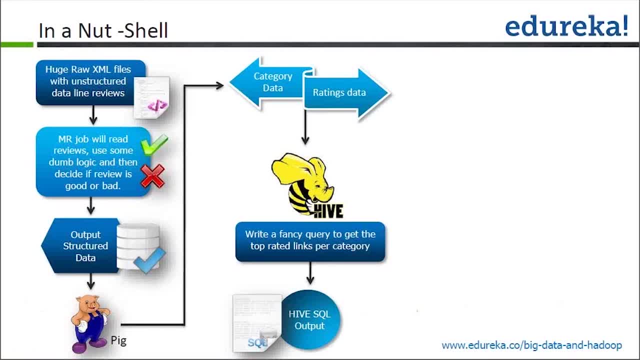 or my sequel, and then your reports connect to that particular database where you put the data and then then consume the data. so in our cases of our data was XML data, so we can very well bring a structure out of that and that data. we can expose it through the 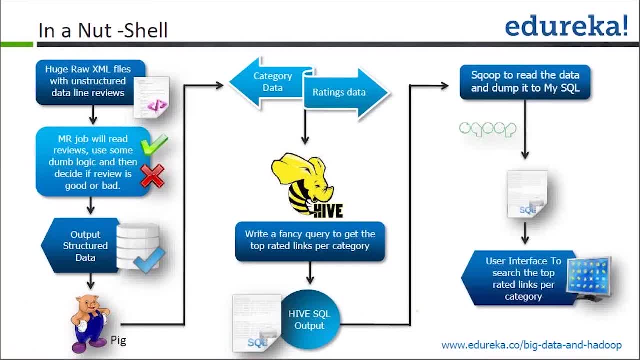 reports, walkthrough. guys, one thing is like you know now, since you have understood about Hadoop, so now you can take a better call, like when you want to go with the MapReduce, when you want want to go for big, when you want to go for hive, how you want to bring the data, how you want to expose the data. right, so all. 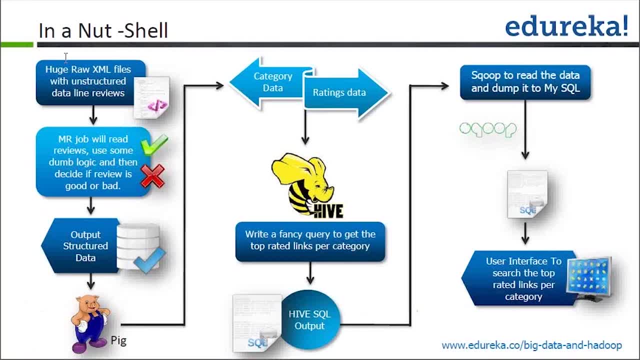 these clarity is now there with you in terms of understanding about the Hadoop system, ecosystem, and you know, are putting all these tools together to solve a, obviously, if a problem in terms of the real world problem. only thing what you have to design is, or more practices like how you will write the logic. so now we have learnt about how to. 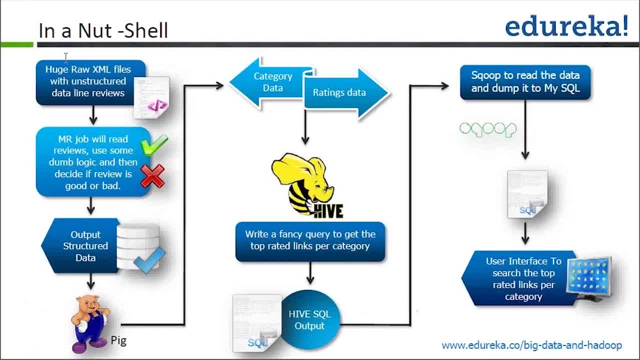 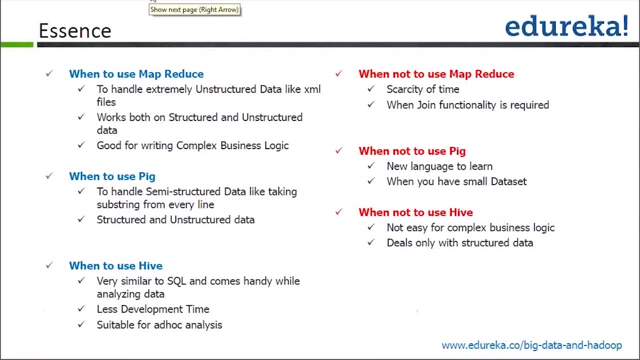 use hive, how to use big only thing based on your business requirement. now you are going to come up with your logic, how you are going to process the data with the hive right, what kind of you know the table you are going to create, which columns you going to create and what type of numbers you are going to do, Che …so in a sense, right. 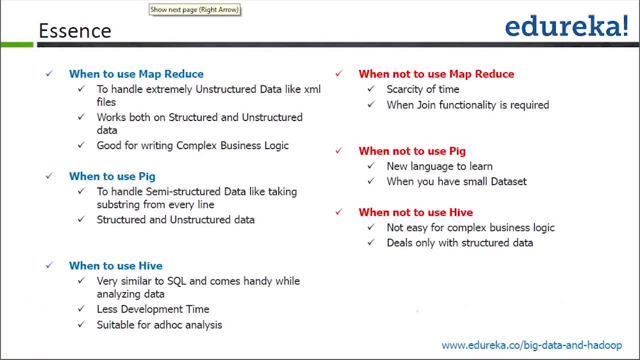 so always, whenever you will come for the Hadoop, you know, designing the solution, you will always have this question: when shall I go for MapReduce, when shall I go for big and when I should go for hive, right? so here is one page slider, guys, one page slides, so that will help you, you know, to basically identify when you should approach. 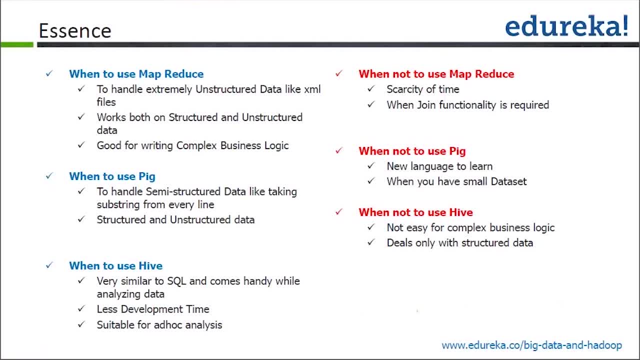 which kind of so? basically, this is a kind of a guideline for you to approach when you when you want to go for MapReduce, Hive and PIC, Okay. so now, when it comes to like, not deciding when you want to go for MapReduce, 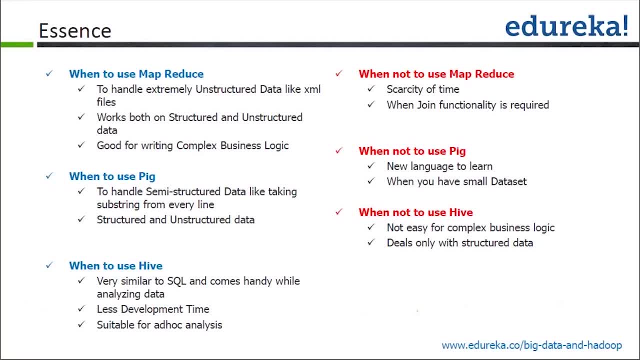 PIC and Hive. here are certain guidelines, guys. So you go for MapReduce when the data set which you want to process is basically alone on such a data, or you know it's like a lot of XML data you have and you want to meaning a structure out of that. 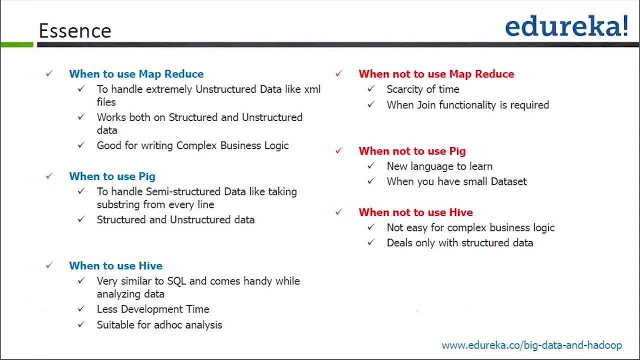 and then you want to process with that case you use MapReduce. Good thing with MapReduce, guys. it's good with both the you know the structure data as well as the uninstructed data. So both kinds of the data you can process here. 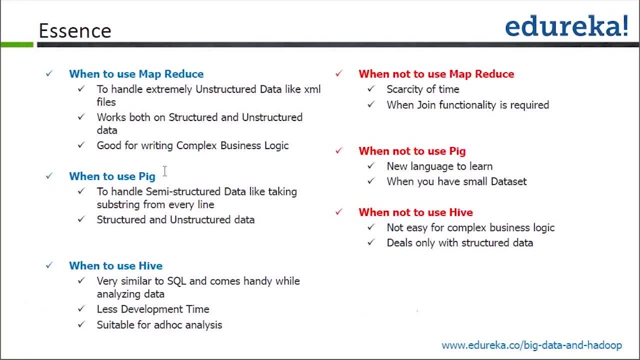 And if you have a very complex business logic and, like you want to do a lot of sorting of the data and you know combining the data, So all those like very highly complex logic, you can do with the help of the MapReduce When you should not use the MapReduce. 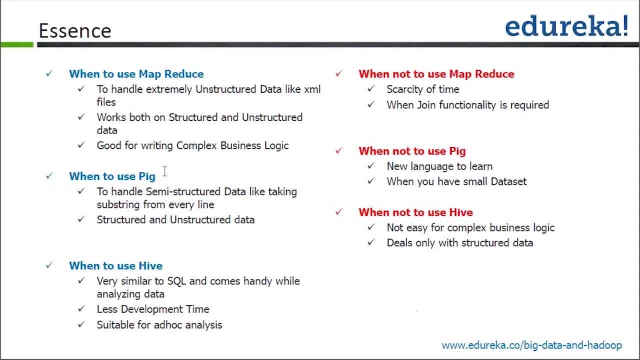 like when you have some kind of a time constraint- you have the. you know the time is not like you know, is like available to do the MapReduce job because it takes time to write the MapReduce program, And when you have a certain like the join of the data. 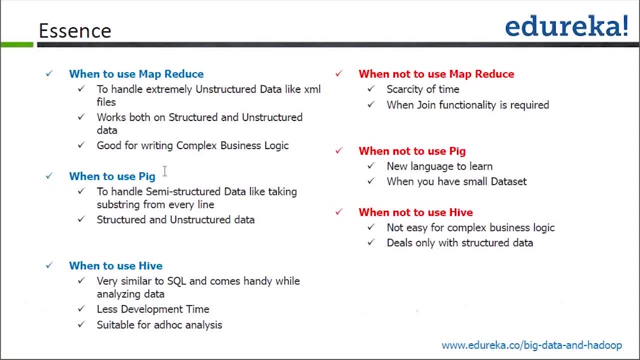 if you remember our discussion about the advanced MapReduce guys, how complex it is to do the join with the MapReduce code because you have to write so many lines of the code to do the join, So that again becomes a challenge here. Case of the pig: if your data is like semi-instructed data, 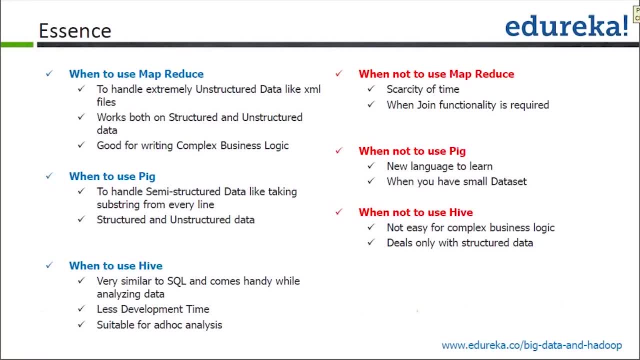 and you want to basically process that data. So in that case you can go for pig. One of the thing is it's a kind of a new kind of the language so that you have to learn. So basically you have to learn pig operator. 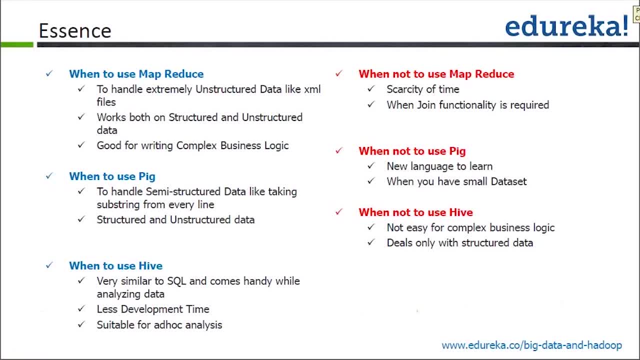 how to submit the data, all the things you have to learn And, in case you know, if you have very small data sets. so in that case again, pig may not be a suitable, because if you have few lines of the code, 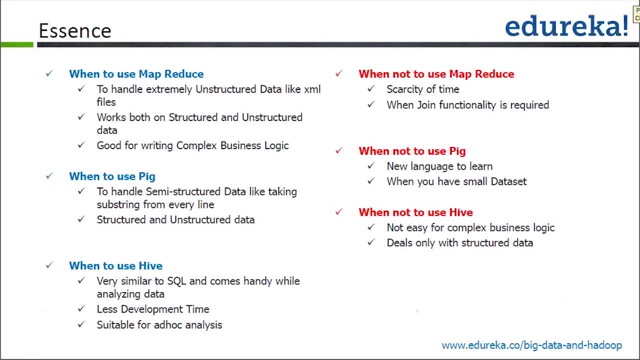 which you will, data which you want to process- pig is starting over the head itself- will be too much than you know what the performance benefit you will get In case of hive. it's very similar to the SQL, So whenever you want to have, you know. 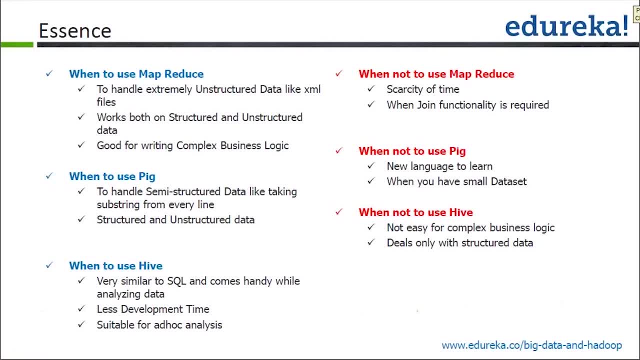 have less development time and you want to do a lot of ad hoc kind of analysis, like, okay, tell me about these three columns, What is the aggregated data? Add two more columns and then tell me, like, what's the aggregated data? 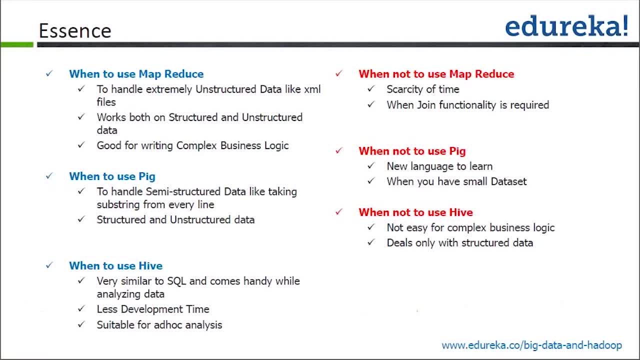 So if you want to have that kind of analysis, you can use hive to do that And you will be able to basically, you know the process data with the help of the hive in a very in a faster way. So that will be basically the less development time. 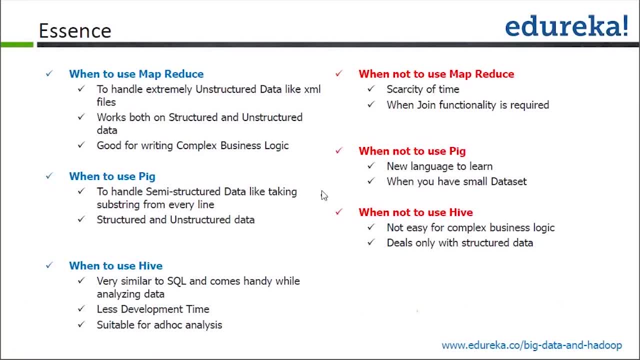 Only thing what you will have is with the hive is like, if you have a lot of sector data or something, you will not be able to do that, And also, you know, if it is like a lot of complex business logic. 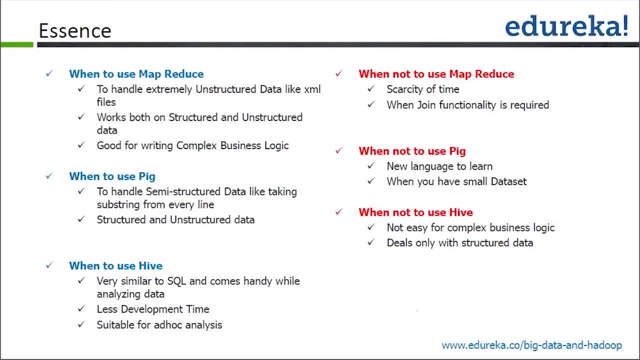 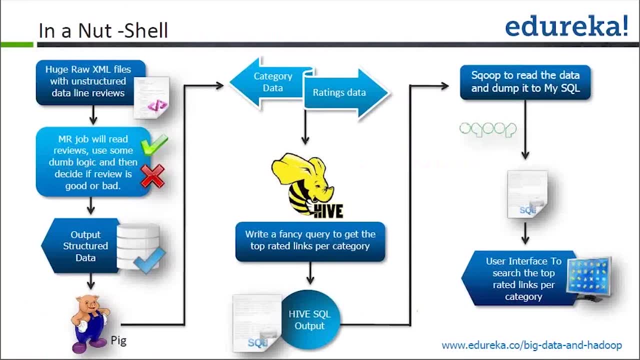 so sometimes implementing that in hive may be challenging. So now, with this right, once you have this particular understanding guys about, like you know when to go for what particular stuff, right, I will share you with the dataset what we have as part of this class of it. 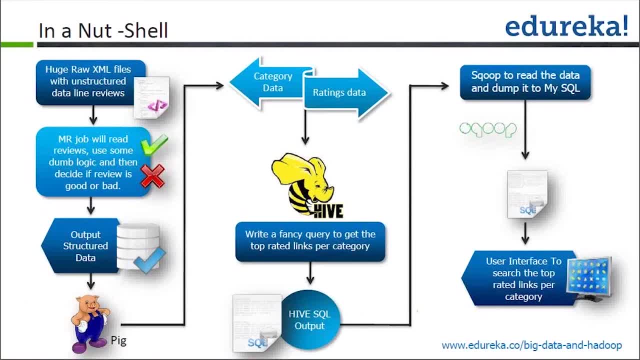 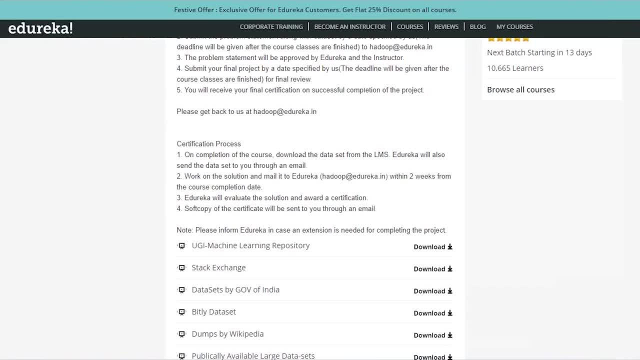 which you can go ahead and, you know, implement as part of the whole the project dataset. so let me get the dataset guys here for you. So this was the LMS access which I was showing you guys. So, once you come here, the big data and how to project. 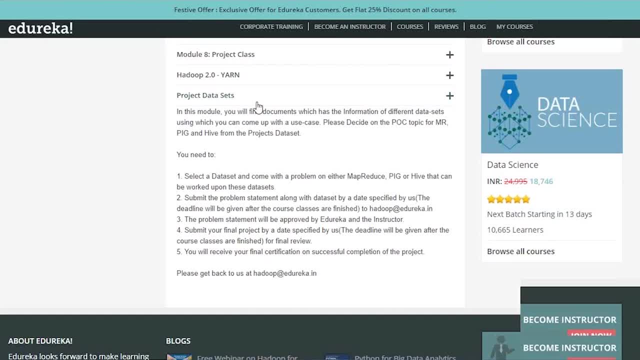 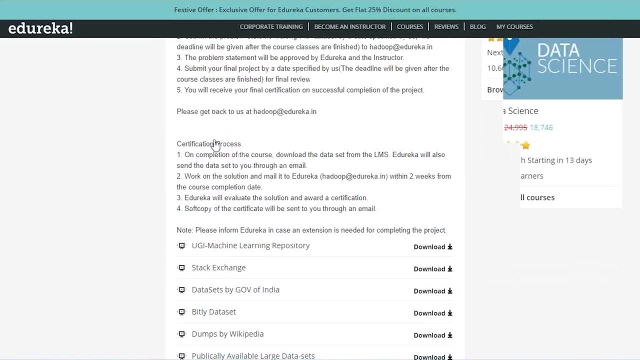 here you get this project dataset. as part of, you know, this last module, you have the project dataset. Once you do this, you see that these datasets will be available And, along with that, you will also receive an email that will have a, basically. 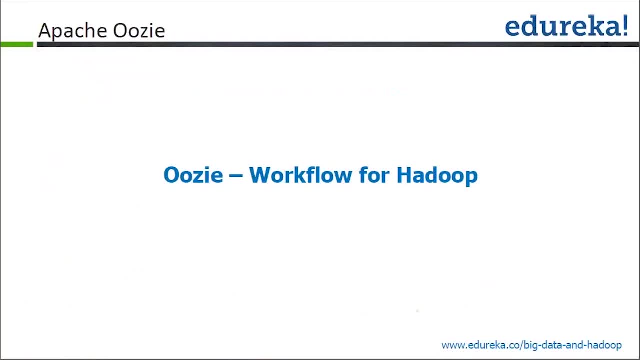 link to download these datasets. okay, So now we are just getting started with the Uzi. So Uzi is something to execute and monitor the workflow in in Hadoop and it critically schedule the workflow, trigger, the execution of the data, based on the ability. 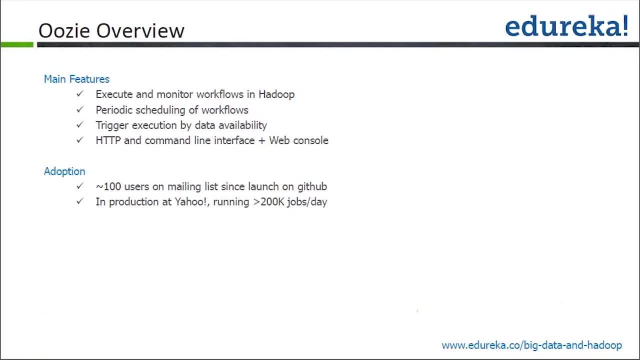 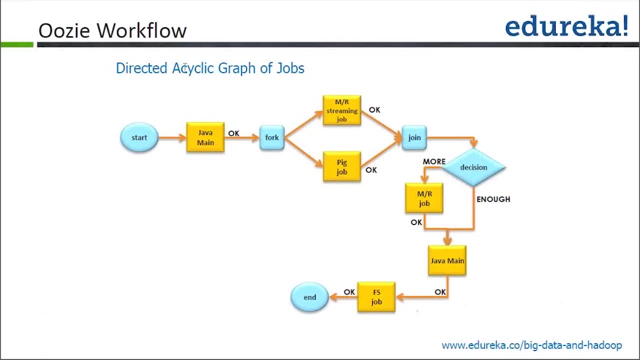 and it can have both the command line and the web interface which can interact with. Okay, So, when it comes to scheduling a job in Uzi. so what you have is you basically created this. you know, DAG, that's called directed acyclic graph. 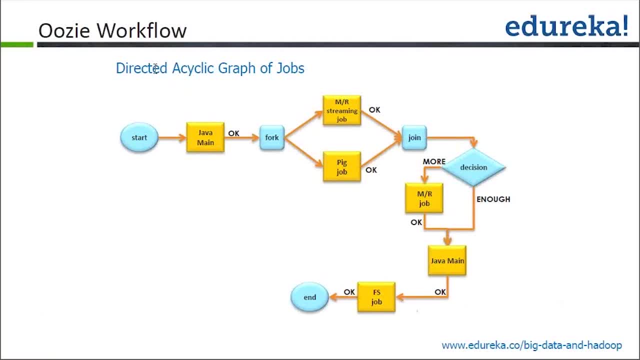 So you did, you decide your workflow based on the different control flow and the action node. So like you have a start and end and kills. So these are the different workflow you have that basically tells, like, from where to start the job, where to stop the job and how to basically, you know, stop a job, in case there 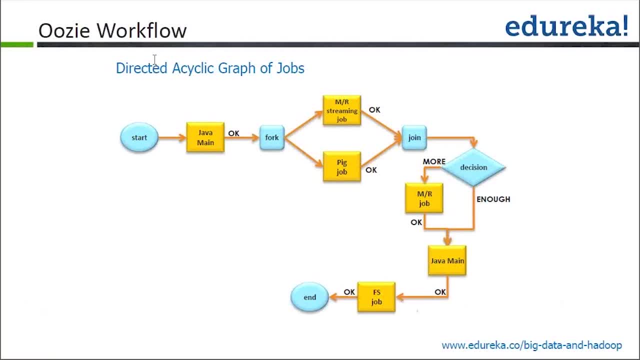 is any failure or something, And then what you have is you have the. you know certain decision nodes like, based on certain condition, you want to go for this particular flow and other flow. So all these are comes as part of the control flow which you have. 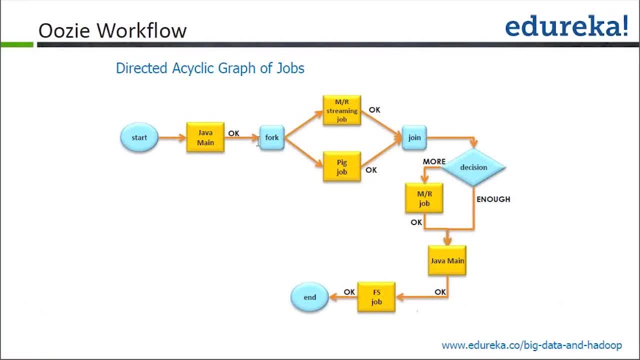 Then you have this fork and join. So if you want to have two sub process to running that, so you can fork that stop process and it will create two that If you want to join these two data set, again you can do the join and you can combine the. 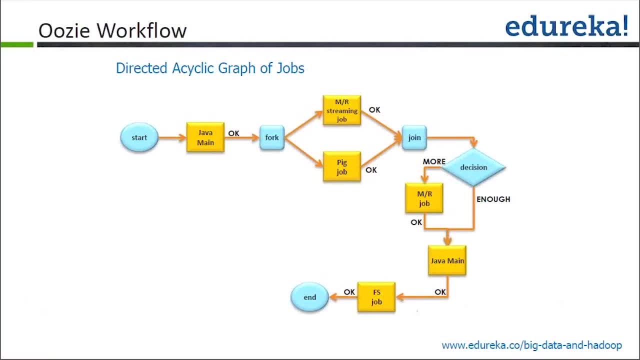 data set, Then what you have is like: apart from that, you have this action node, So that's basically do the actual execution of the job. So like suppose, if you want to run the MapReduce, you want to run PIG, you want to run Hadoop. 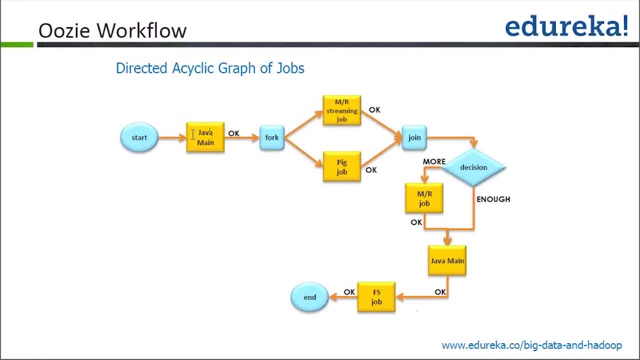 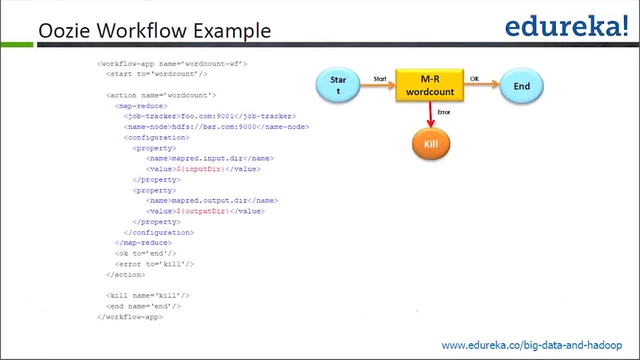 So all these action node, you can use it that like, suppose, if you want to read the file, you want to send an email, So all those kind of this stuff you can do with the action node. So how you, How you write this whole workflow, guys, is basically you create a XML file. 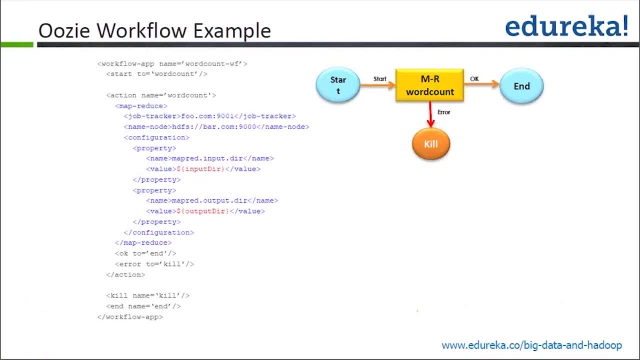 So Uzi, basically it's having its own language called HPDL. So Hadoop is like you know, you define the whole process definition language. So that's nothing but a kind of you know the XML kind of the file where you specify what job you want to run, what is the input directory, what is the output directory, what is the? 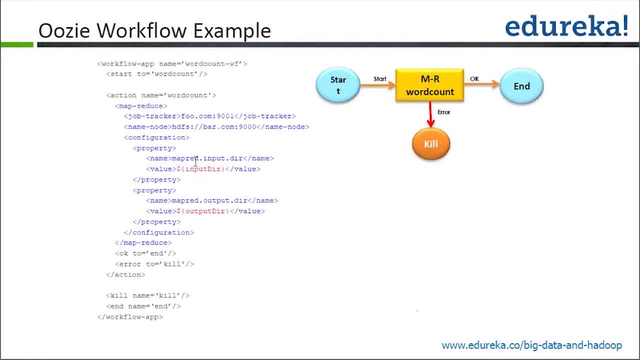 starting node. what is the MapReduce processing node? So, based on that, you know. So you take this data set and you process it here. Okay, so you have this XML file right. So what you can do is like, suppose, if you want to deploy a simple MapReduce job, 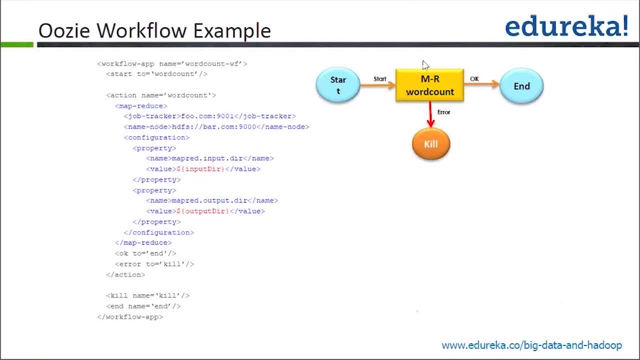 So you will have a start node where the whole processing will start. Then you will have this MapReduce word count like: so that's where the action node that will execute the MapReduce job. So it knows like it has to create a new directory or, if it's active, as you're saying, go ahead. 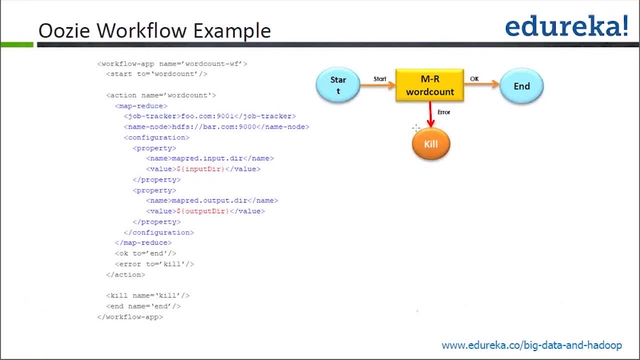 and delete the directory, Right. So all those things. So these are part of all these: action node, the MR unit, sorry, the MapReduce node which you are using, the action node which you are using, And then, in case there is any failure, so like if the data set is not available, in that case, 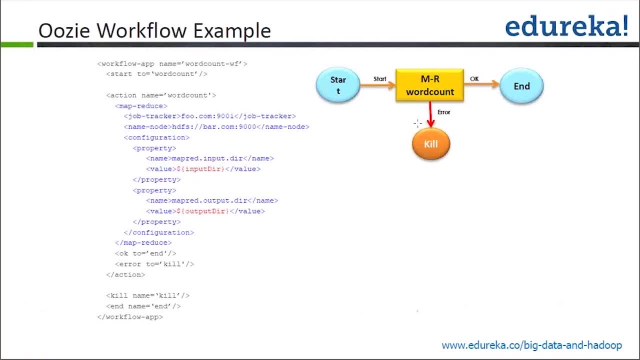 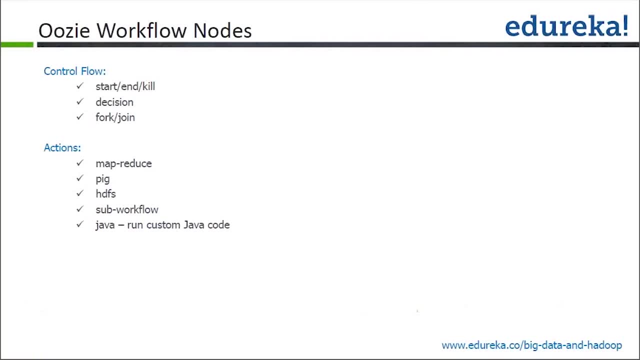 job will fail and you will basically send a kill signal and once the processing goes, it will reach the end node and that's where the whole workflow will complete. Okay then, these are the workflow you have, guys, So, and the nodes which you have. So you have the start and then kill. 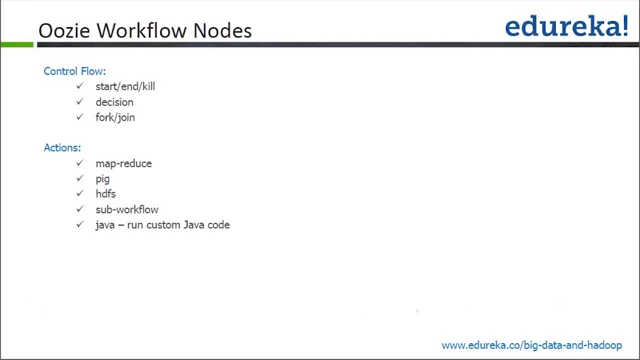 So that's basically the control. Then you have the decision boxes like: so that's where you decide, like whether to go with this particular flow or the alternate flow, And then you have the fork and join where you want to create two sub flow and join the. 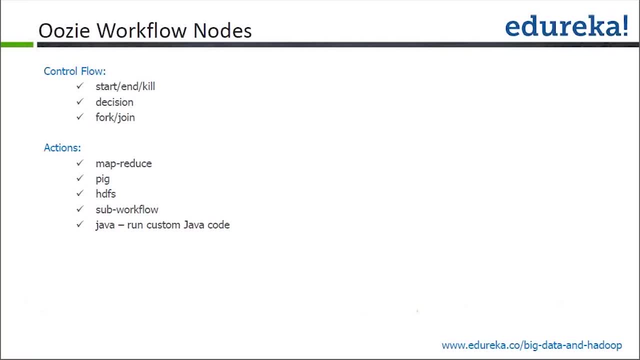 data set Actions. you have the MapReduce, pick, HDFS, any kind of you know custom Java code you want to run. So all those things you put it as part of the Java or as part of the action node. So how you deploy this Uji stuff, guys? 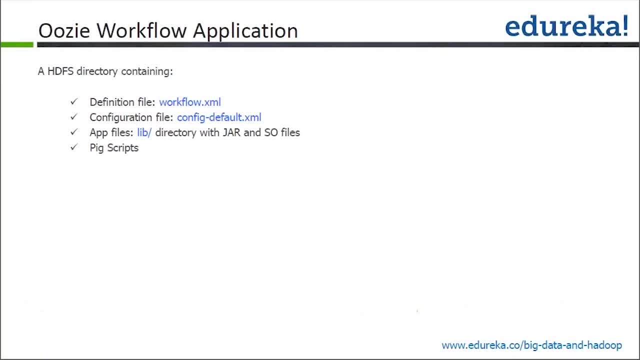 So you basically create this workflowxml file and you create certain configuration file, like you want to like have these things parameterized, not like hardcoded in the workflow, like input directory or output directory or any other parameters, like if you want to move from dev to production. 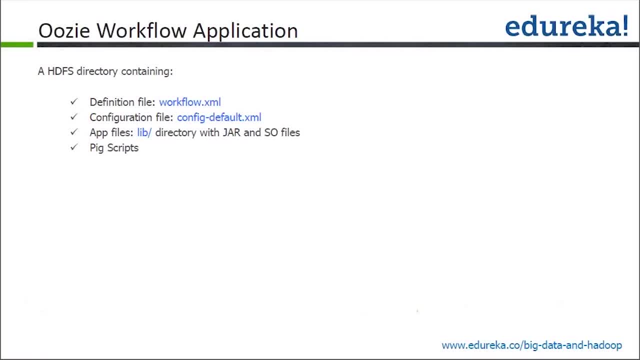 So all those things should be part of the configuration file. So once you have all this one, so you move all these files into the lib directory along with the jazz file or any other you know supported files which you have for your program, and then any other big high. 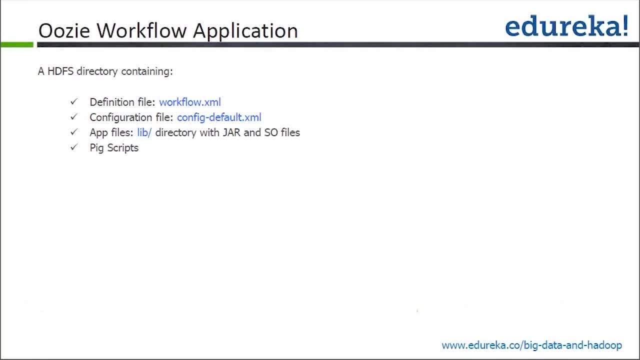 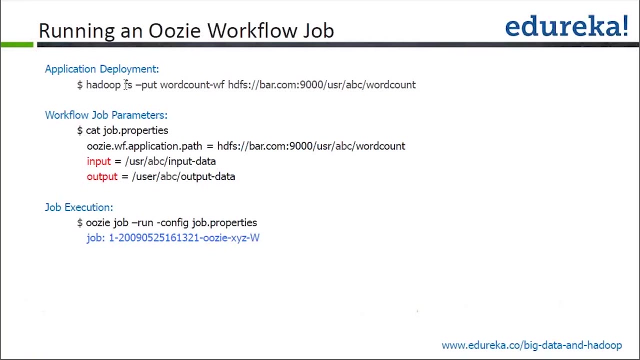 So whatever the script you want to run, so all those things- you move in inside the HDFS and then you submit this job from the command line and then it will start executing that. So how you do that is: you basically have this Hadoop FS app input and then you specify what. 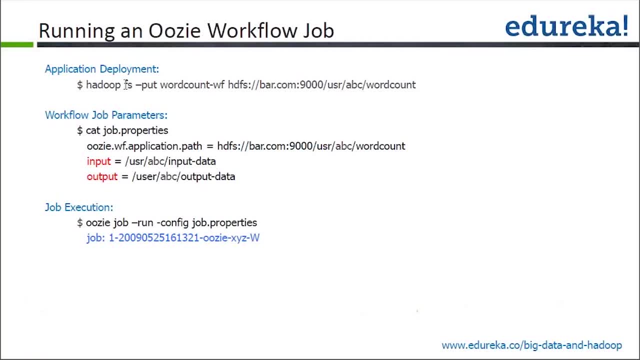 kind of you know the configuration file you have. So, based on that configuration file and the xml file, you submit the job to basically deploy to the Uji server and Uji have its own database guys, where it maintains all the data, All these jobs, and you know the status of the job. 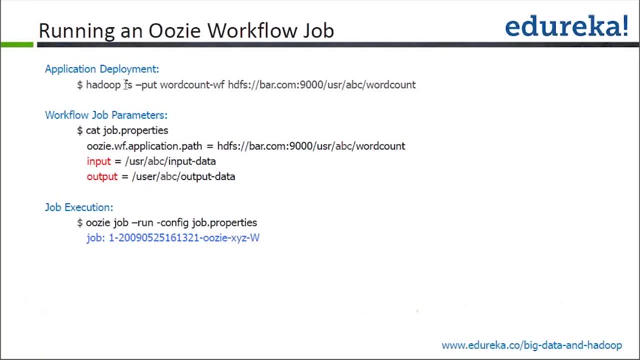 So once you do that, it will basically get all the information about the job property, like what is the input data set, output data set and whatever the workflow you have put in the xml file and based on that, it will start running the job. So you will get a job id. so by using this job id you can always track that, how the jobs. 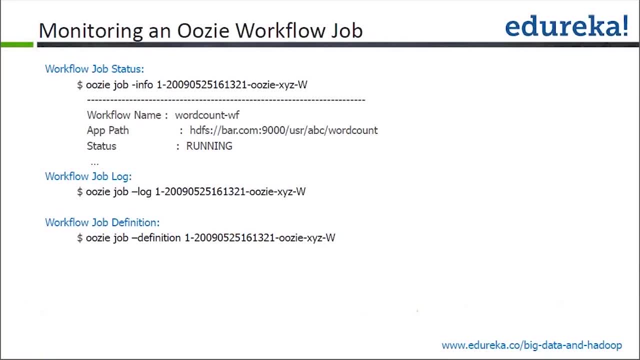 are basically progressing inside the Uji. you know control flow so you can see the information about the jobs. So once you submit Uji job info and you can give the job id, it will show you the status, like whether the job is running, killed or, you know, completed successfully. right. 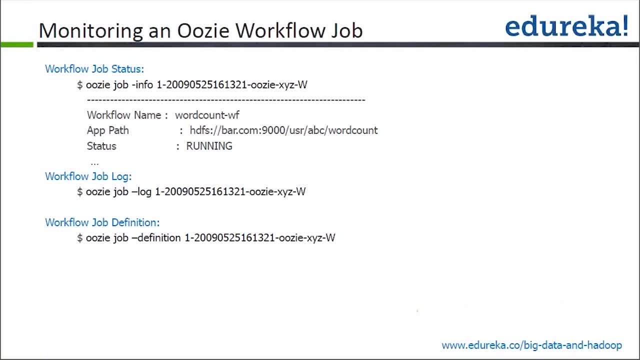 So all the jobs will have its own log file as well, so you can see the log in case of there is a failure, you can basically, you know, look into this log and debug this stuff. Okay, so, in terms of the flow, how this happens, so Uji has, once you submit a job, Uji has a. 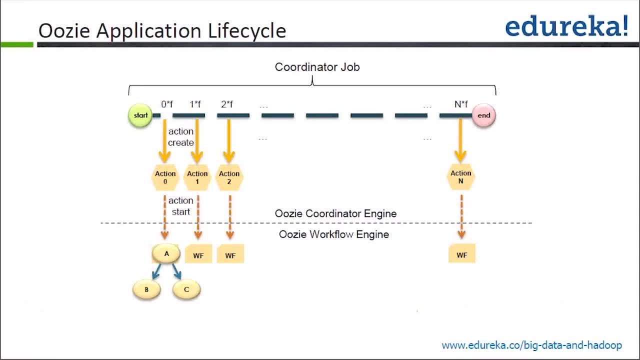 coordinator job. so what that does, is it basically? you know it basically takes care of the whole flow. So in a flow you will decide like, okay, first I want to do the map, reduce processing, then I want to do these set of the peak processing, then hive, and then finally I want to scoop. 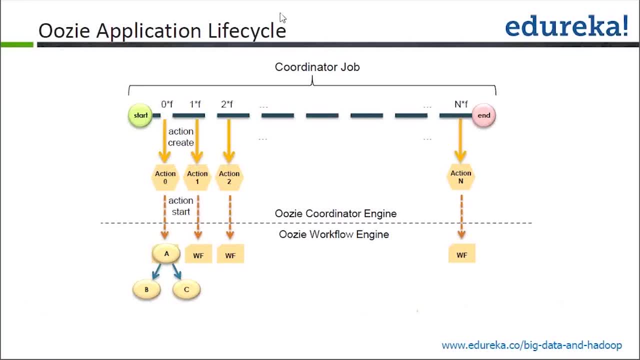 the data right. So, based on the, whatever the logic you are writing, based on that particular logic, it is going to keep moving your the flow from the start and till the end. So as soon as it will encounter the end node, it will basically complete the whole workflow. 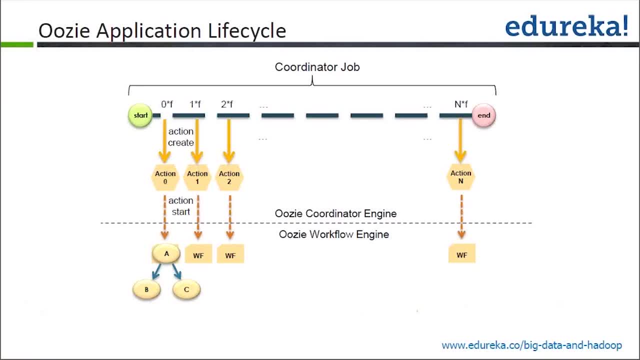 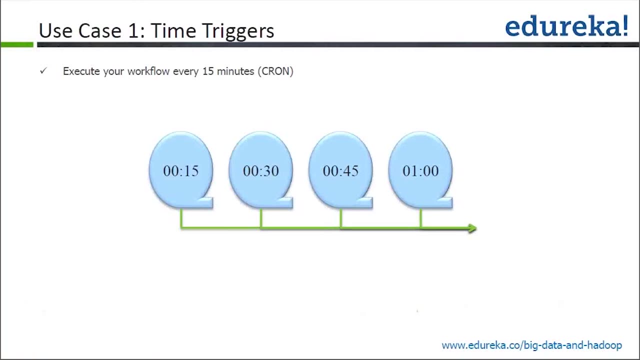 And as the flow is moving, you will have the Uji workflow engine That will basically keep executing those tasks and you know it will be taking the action like whether to run the big job, higher job, so that that particular stuff will be done by the Uji framework. 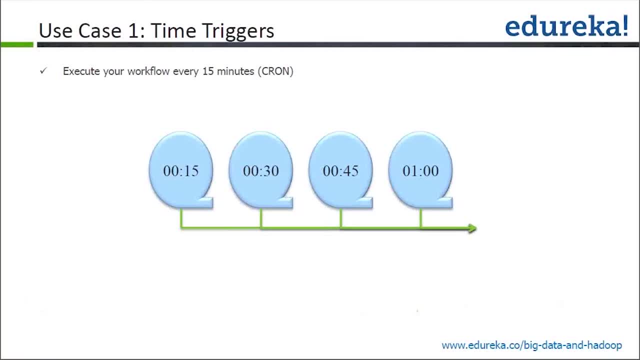 Now, when it comes to basically, you know schedule the job inside the Uji framework guys, so you have the different way how you can schedule the job so you can have the workflow like which can be done every 15 minutes, kind of thing, So like. 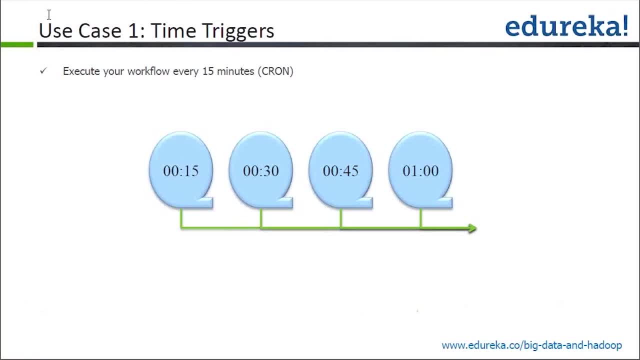 You can have like a job which you can schedule. let's process that every 15 minutes So you can schedule those kind of the jobs inside Uji. So all you have to do is you have to define the frequency as 15 and, based on that, every 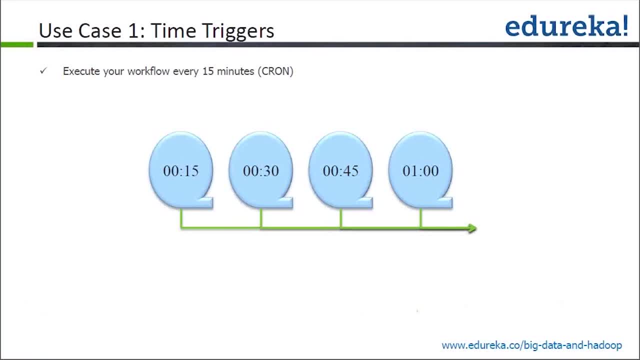 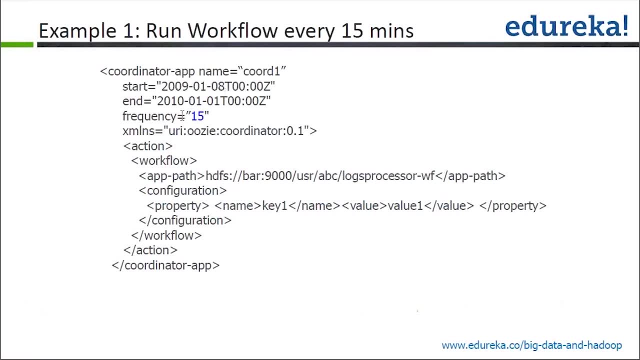 15 minutes based on the starting time it will. it will start running for the next- you know next- one hour, like every 15 minutes. it will keep running, So you can have your start time and time and then you can give the frequency and it will. 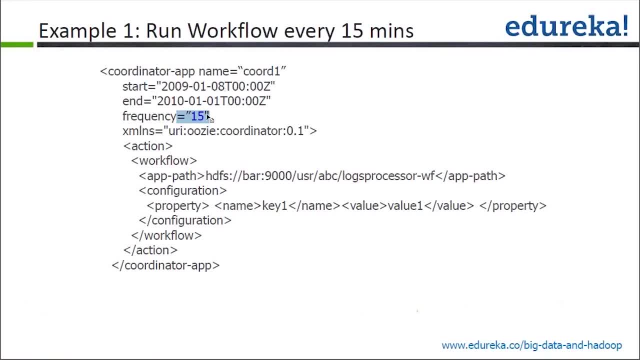 keep running that particular, the workflow which you did, which you submit. it will for every 15 minutes, kind of thing. Similar way, if you want to have like scheduling, like based on the availability of the data set, so in that case what you can do is like you can give a particular folder where you 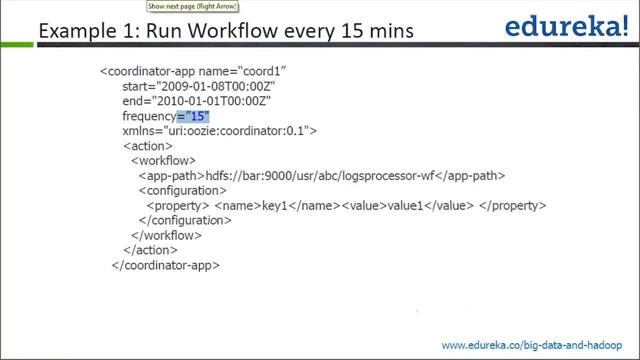 want to look for file, like, suppose, if your file is getting delivered from some some kind of third party system and based on the file system where, like you have, you want your application, like every hour, to connect it to it, and then you know, run the job. so what you can do is 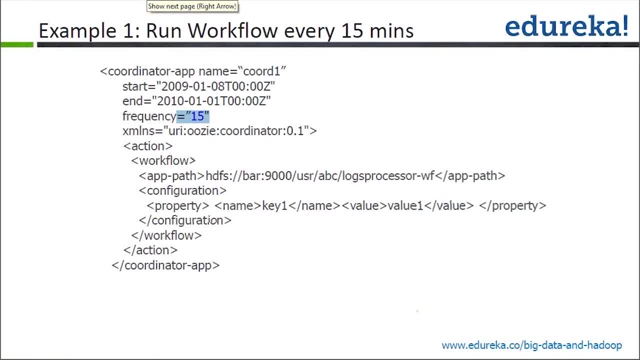 you can schedule that for every hour and once you should do that every hour it will connect to that particular job. So if you want to have a directory, look for the ability of the data set. if the data set is available it will do the processing. otherwise it will wait for the next another hour. it 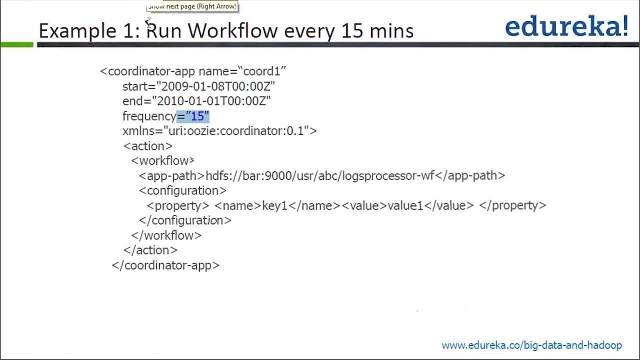 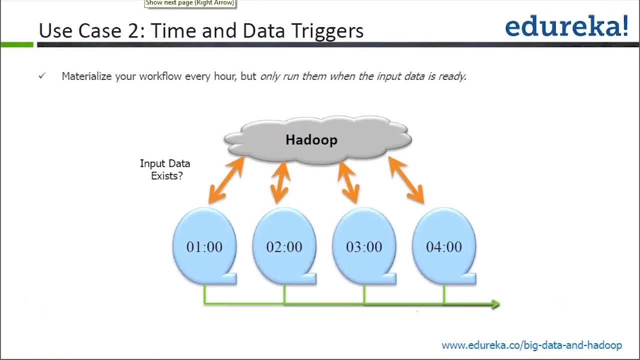 will again pull for the data set and then it will do the processing. So these kind of the scheduling also you can do with the help of, you know, the Uzi. So for that all you have to do is you have to define what is the input data set directory. 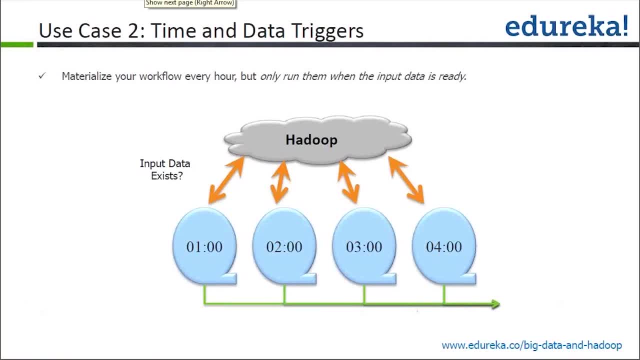 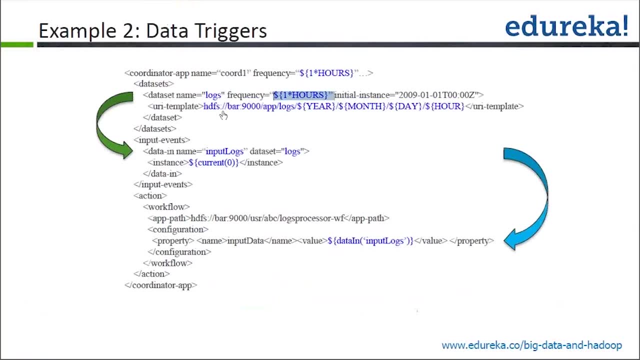 which you want to basically pull and what is the frequency you want to basically go for. so, based on that, like every hour to hour, you want to do that. So, based on that, it will be the data set. Then you go ahead and you know, look for that every hour. and this is the directory which 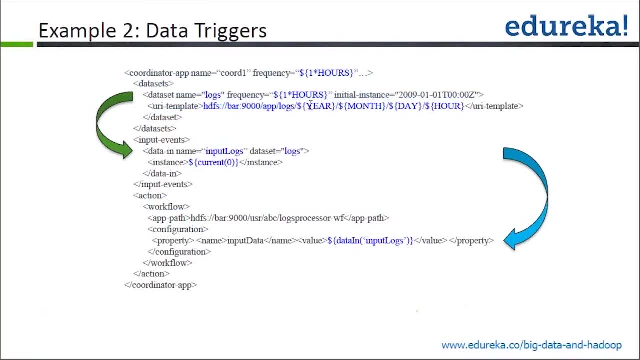 you will satisfy. So generally in Hadoop what you will have, guys, is this: you know the year, month, day and hour kind of the directory structure you have, so like every hour you can ask like to come and look for this particular log and based on that, if there is an input log or some kind, 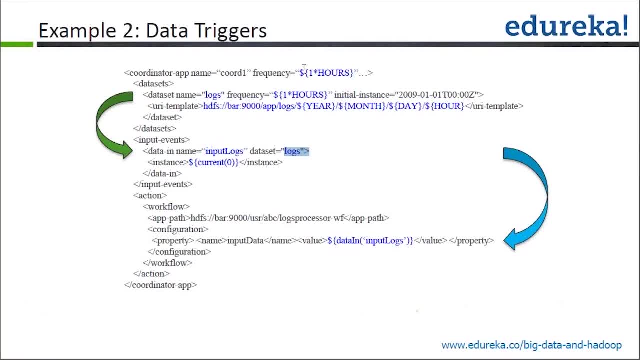 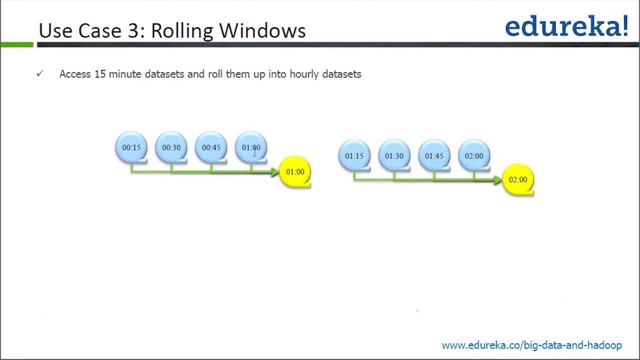 of the data set like logs are there, it will go ahead and you know, look inside the directory. Then also you can implement like suppose, if you want to aggregate the data and then you want to run like your data is going to come every 15 minutes. 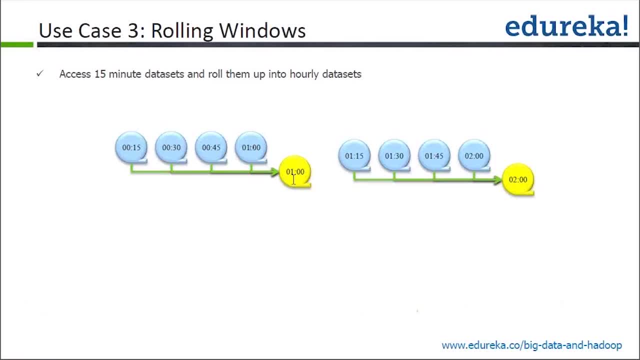 That you want to combine them together and you want to process every one hour kind of thing. So that kind of the rolling window implementation also you can do with the help of the Hadoop. So what you can do that every one hour and it's processing, it can go back to last you. 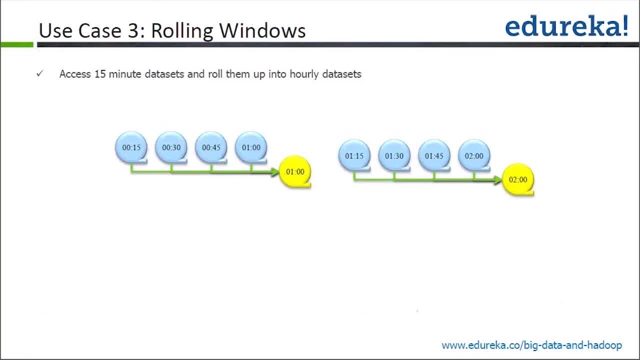 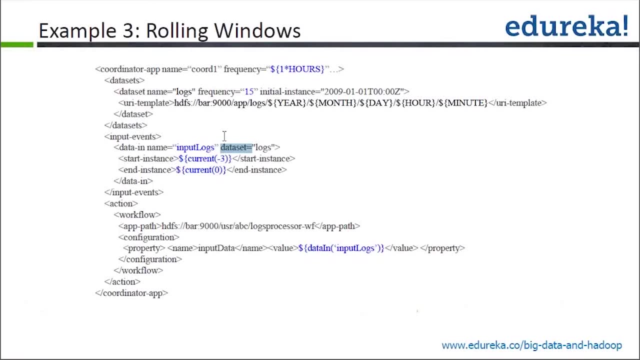 know the four instance, whatever it has, and then combine that and read the data. So what you can do is, starting from current zero, you can go back to the current three instance and then, based on that data set, it will combine the data and, like every time, 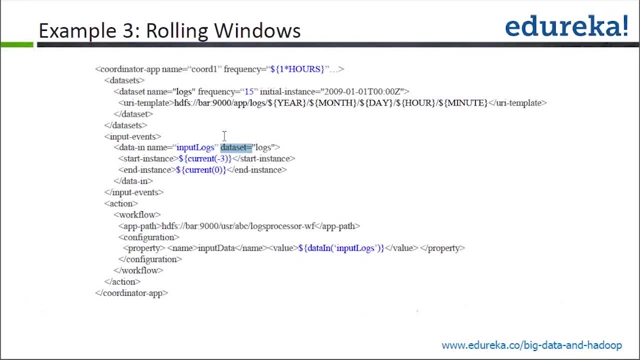 you want like tell me, like last 24 hour, what is the? you know the numbers in terms of the data. What is the numbers of the top 10 URL? or last 10 minutes? what the URL? So, based on whatever the window you decide, it will process the data set and it will give. 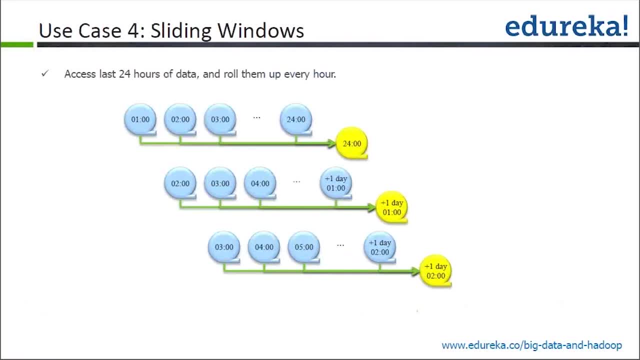 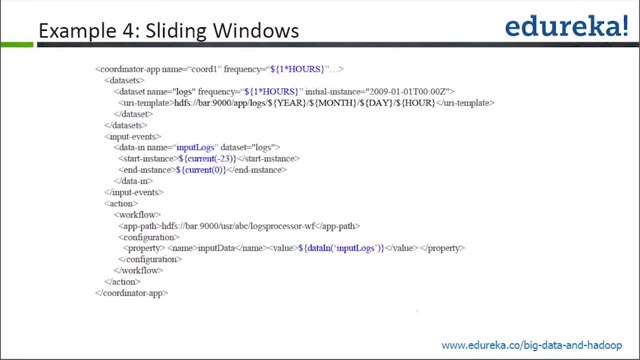 you the output That's every 24 day, one day kind of thing you can. you can get this sliding window as well, So like if you have like every 24 hour, you want to process it every day, like last one day of the data you want to process and see, so you can go: current minus 23, so last 24. 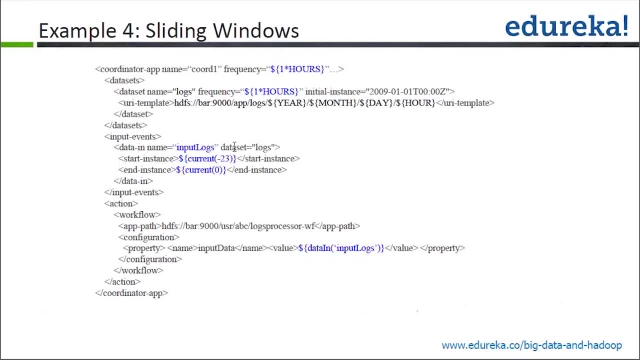 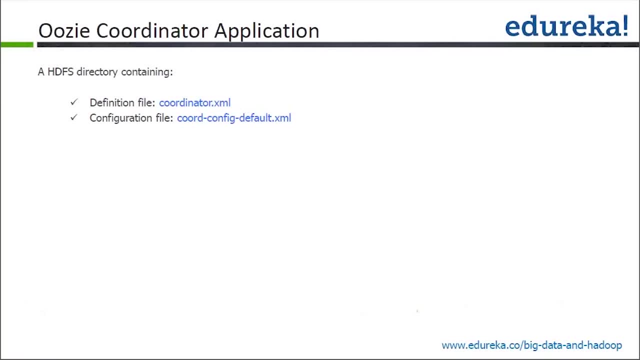 hour. it will process that and give it to you. Okay, so these are the different ways how you can schedule your job. so have you guys used the scheduling tool guys to deploy your jobs in production? So now, when it comes like once you deploy the jobs, right, well, one thing is like: if you 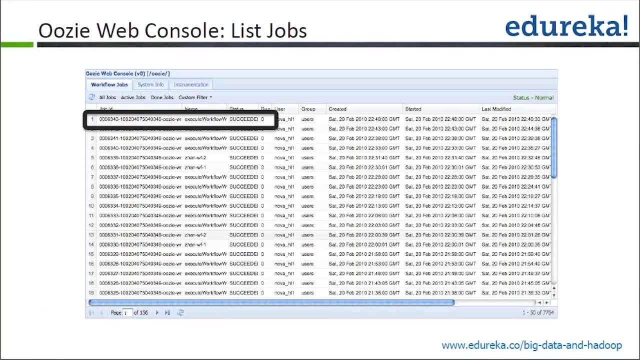 want to see the status of the job. what you can do is you can use this Uzi web console. You can use the Uzi web console. You can see that the job is ready. You can see that the job is ready data. So, by using this Uziweb control, what you can do is you can give these URLs to your 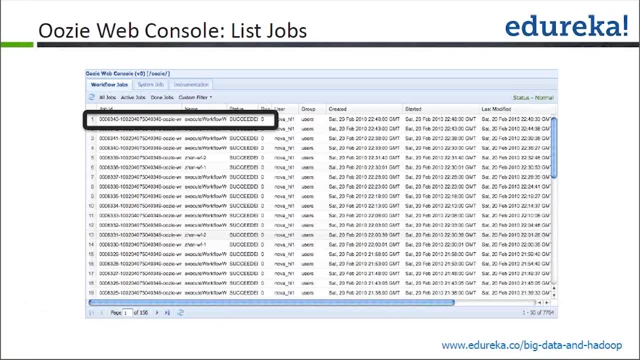 production support team and they can basically monitor all your Hadoop deployment with the help of these URLs and they can see if there is any failure. it will basically show it here in this particular URL so that they can monitor the job and in case if there is any failure. 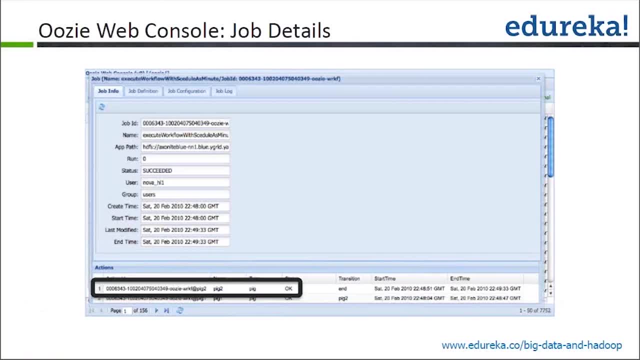 they can get more details about what kind of failure it has and why it has failed. So all those things you can deep dive more in the URL and you can see the details, like what time it started, how much time it took. so all those kind of details you can see from the. 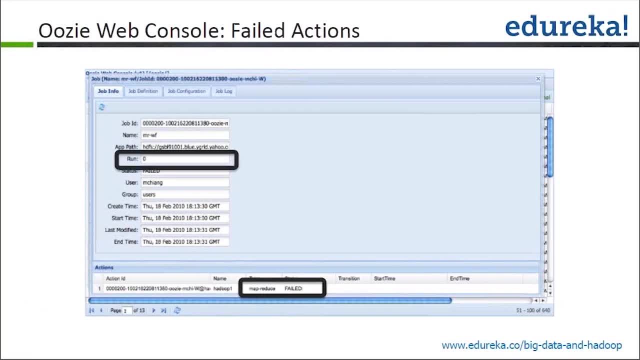 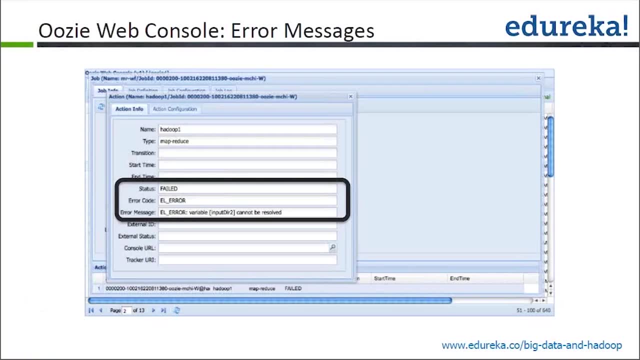 Uziweb URL. so that's what, guys, how you will deploy all these jobs inside the URL so you can monitor the URL, the job status, both from the web interface as well as from the web interface, the command line interface as well. okay, so now, with this case, let me share you. 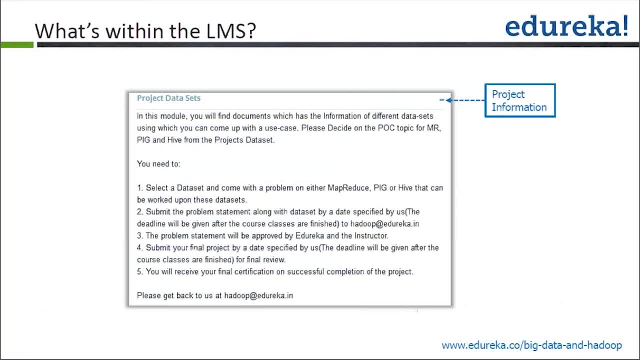 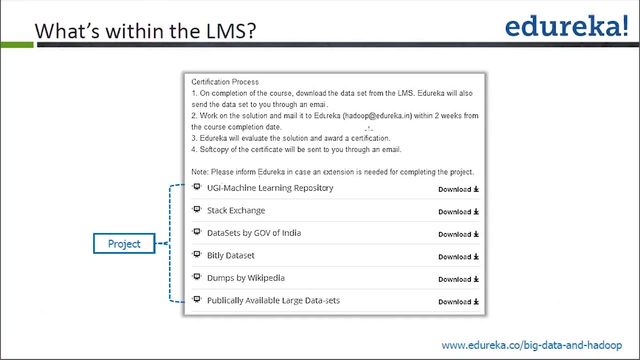 some more details here and based on that, you know, we will conclude this particular module. so one thing is about the data sheet. so all the data set is available in LMS, so you can access these data set very well here, guys. so what you can do is you can get this data set and you can start implementing this project.